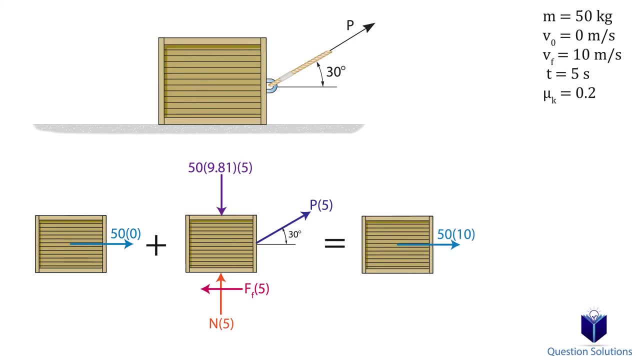 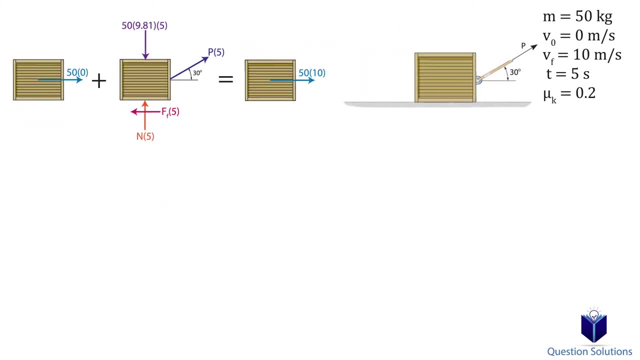 the final momentum diagram, which is with final velocity. in our case that's 10 meters per second. So that's mass times, final velocity. Now we can write our equation for impulse and momentum and we will assume up and to the right to be positive. First we will consider the 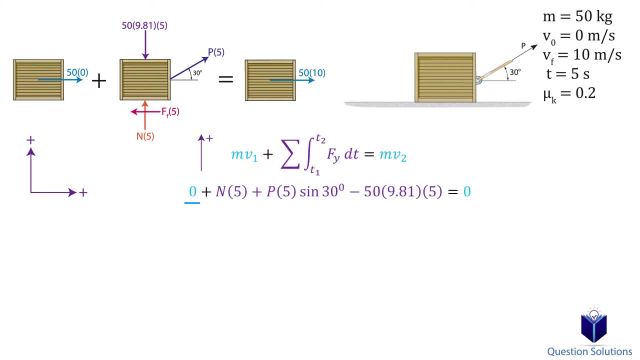 vertical direction. Our initial momentum is 0 because the box is starting from rest. Next we have the impulses, which means we consider how long each force affected the box for the span of our question. In other words, the box moved for 5 seconds. So what forces? 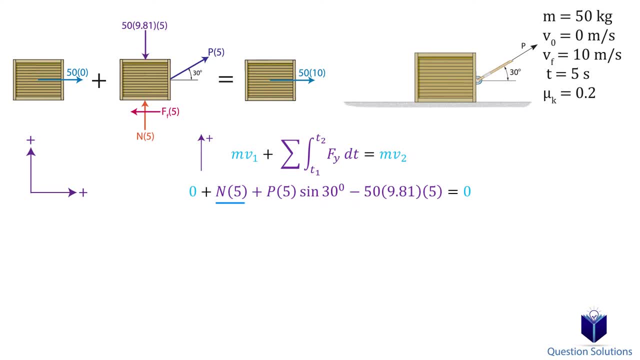 affected it during those 5 seconds. So we have the normal force multiplied by 5 seconds, the y-component of force, p, multiplied by 5 seconds and the weight multiplied by 5 seconds. Remember that's negative, since we chose up to be positive. 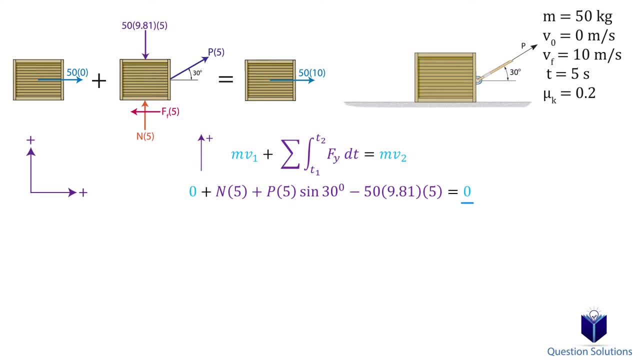 All of that is equal to 0 because the box is not moving up or down in the vertical direction. We can isolate this equation for the normal force and then write another impulse and momentum equation for the horizontal movement. As before, the box starts from rest, so initial momentum is: 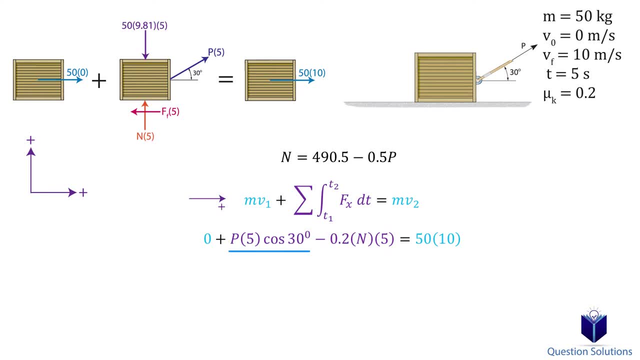 0.. Then we have the x-component of force, p, multiplied by 5 seconds, and the frictional force, which is the coefficient of kinetic friction, multiplied by the normal force multiplied by 5 seconds. Then all of that is equal to the mass times final velocity, which is 50 kg multiplied. 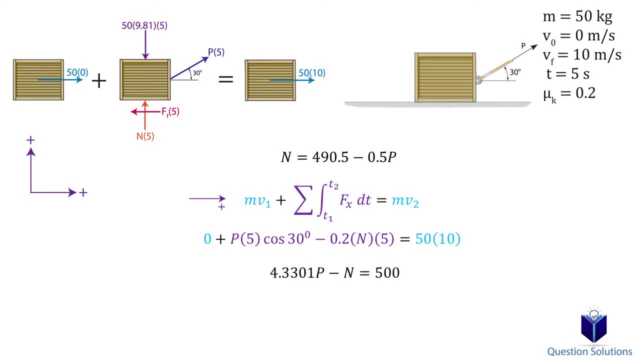 by 10 m per second. Let's simplify this equation. We have two equations with two unknown, so let's solve them. That's our answer. Let's take a look at this problem where we need to find the speed of the crate when T equals 4. 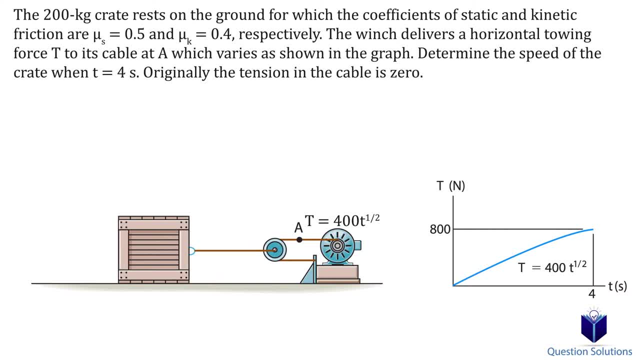 seconds, We're given the coefficient of static friction, which means we will have to calculate the time needed before the crate starts moving. The pressure goes to our x-component, theいう gear carriage speed, which means we need to find the craft's speed when t equals 4 seconds. The volume and the number of stages do not vary from a simple equation to a simple equation. The critical capac90-ambient coefficient is just the number of seconds instead of the moment-. Louise Williamsgetz, but not the identical coefficient, which means that we have to plate each Ray jóvenes and put the potatoes together. 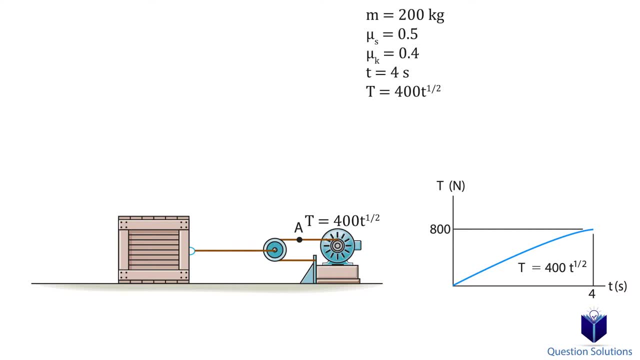 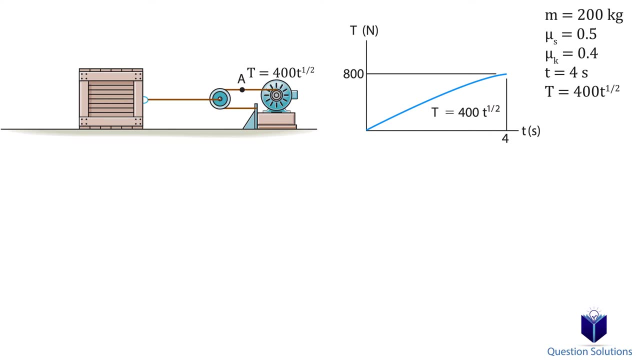 started to move. Think of it this way: the friction will keep the box still until the pulling force can overcome it. So how long did it take before that happened? To do that, we can write an equation of equilibrium. Let's draw a free body diagram showing the forces. 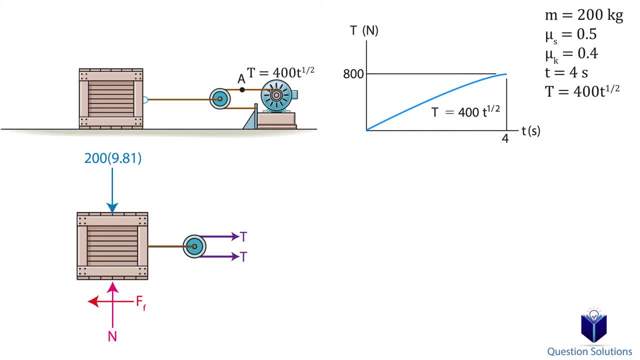 affecting the box. One thing to note here is that at the pulley there is actually two towing forces. It's one single rope being pulled by the motor, which creates equal tensions on both sides. So let's get started with our equilibrium equations. Remember the box. 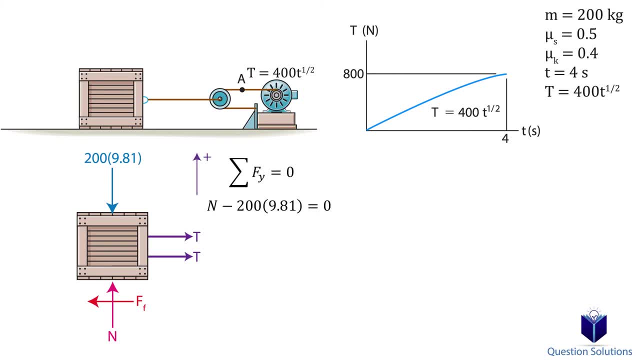 isn't moving, but it's on the verge of moving. Let's write the first equation for the vertical direction. We have the normal force and the weight, which is equal to zero. This allows us to find the normal force. Next, an equation of equilibrium for the horizontal forces. 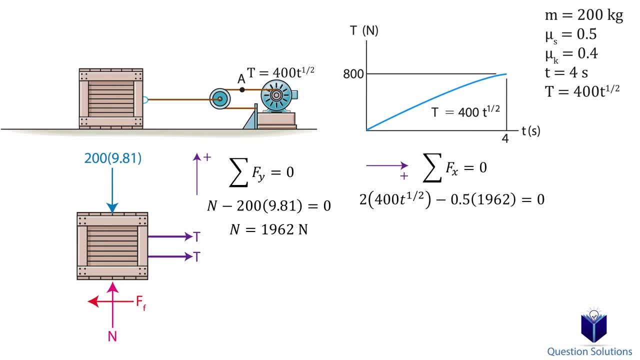 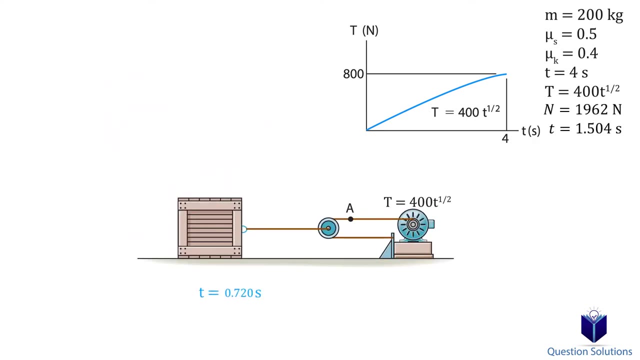 We have the two towing forces and then we have the frictional force. Remember, frictional force here is the coefficient of static friction multiplied by the normal force. When we solve this equation, we get the time it took for the box to start moving. So we get 1.504 seconds, which means that's how long it took for the 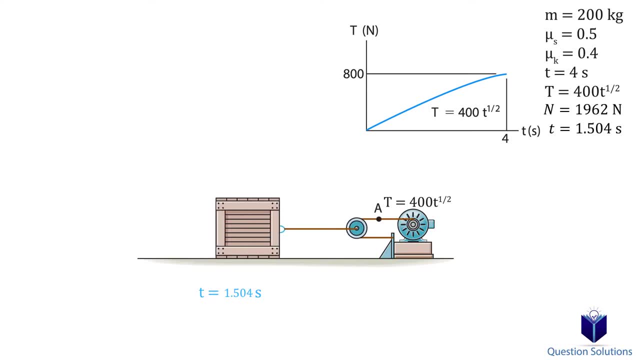 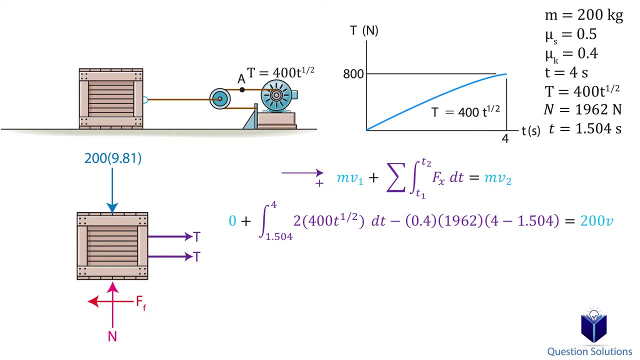 box to move, overcoming the static friction. Now that we figured that out, we can move on to an equation of impulse and momentum. The initial momentum is zero because at exactly 1.504 seconds, the box is just about to move. Then we have the impulses, We have the towing. 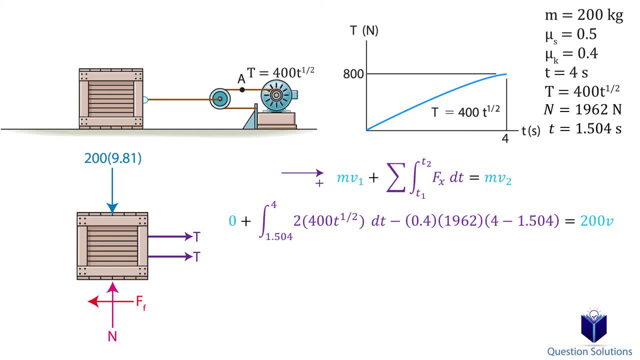 force and since it is not a constant, we do need to integrate it. This is where the time comes into play. So the box started to move at 1.504 seconds, which is our lower bound, and for the upper bound it's 4 seconds, since that's when we want to find the velocity, Don't forget it's. 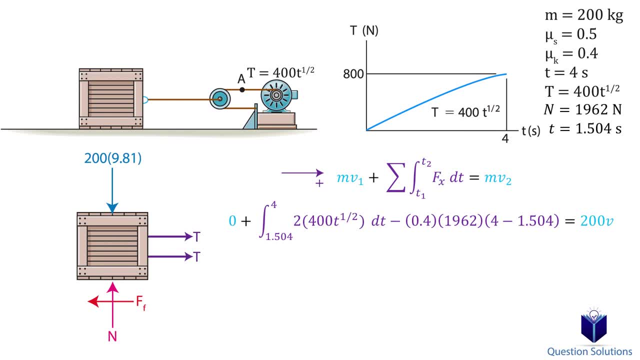 two towing forces as well, We also have the frictional force, which is kinetic friction. now, since the box is moving, That's the coefficient of kinetic friction multiplied by the normal force, multiplied by the time the box moves, Which again is 4 seconds minus the time it took for the box to start moving Then on. 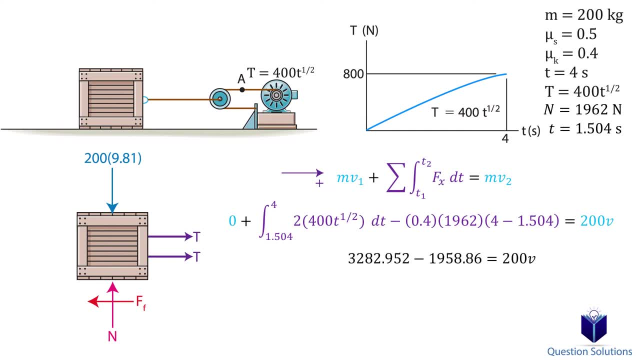 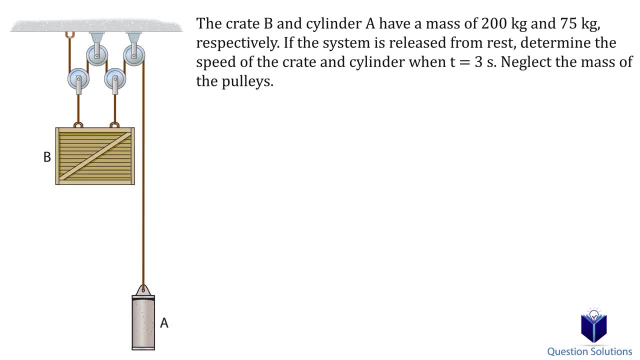 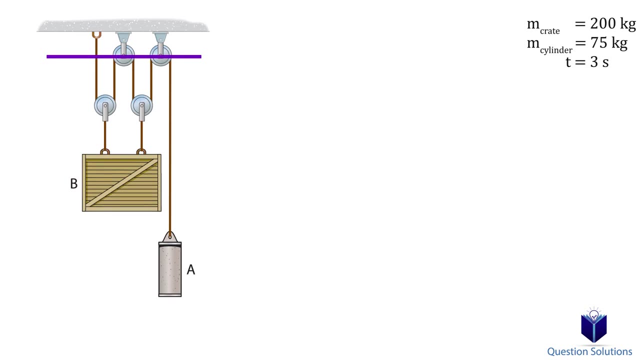 the other side we have mass times, final velocity. Let's solve and that's our answer. Let's take a look at this example. In this problem we need to find the speed of the crate and the cylinder when t equals 3 seconds. Let's start off by first drawing our datum on the top. 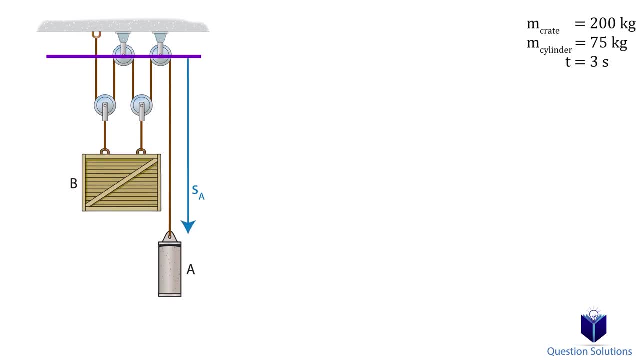 pulleys For our position coordinates. we have SA and SB. Now we can write an equation to represent the cable. It's one cable, so we only need one equation. We have SA plus 4SB, which is equal to the total length. Let's now take the time derivative to get an equation. 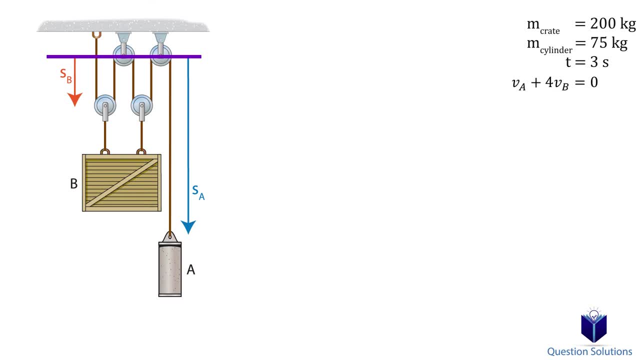 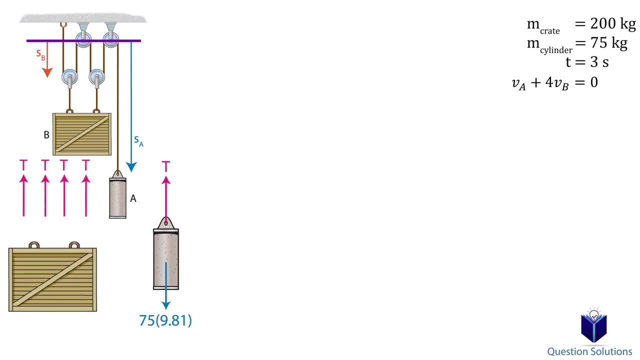 for velocity. Now we can set the velocity equation to the side and move on to equations of impulse and momentum. First we will draw a free body diagram for the cylinder. We have the tension and the weight. Next, a free body diagram for the crate. We have four cables. 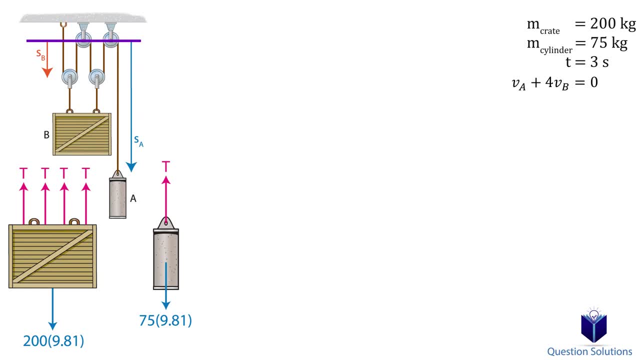 and we have the weight. It's important to note, since we drew our position coordinates downwards, we are assuming both the cylinder and the crate will have a velocity downwards. Now let's start writing our first equation, first for the cylinder. Note that we are only 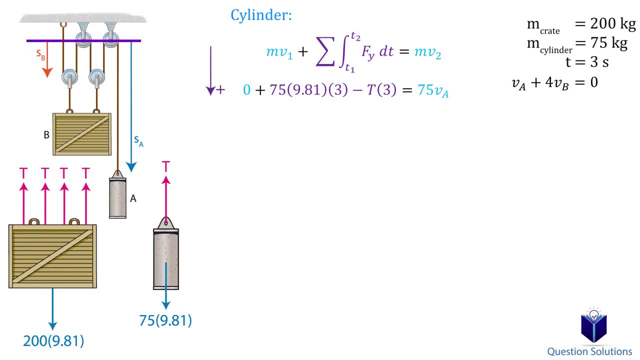 considering the vertical movement, and that downwards is positive, So the initial momentum is zero, since the system is released from rest. Then we have the impulses, which includes the weight multiplied by 3 seconds, and then tension multiplied by 3 seconds, So the momentum 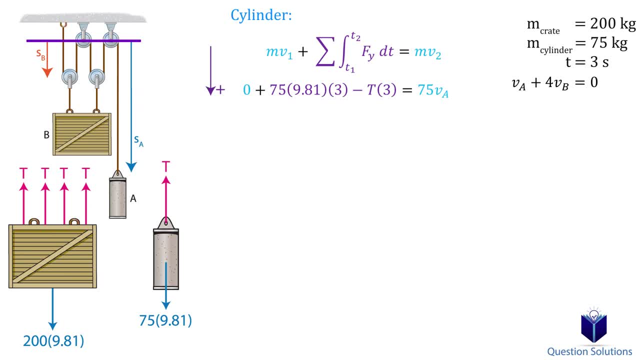 is zero, since the system is released from rest. Then we have the impulses, which includes the weight multiplied by 3 seconds. All of that is equal to the mass of the cylinder multiplied by the velocity. Let's simplify the equation. Let's set it aside and move. 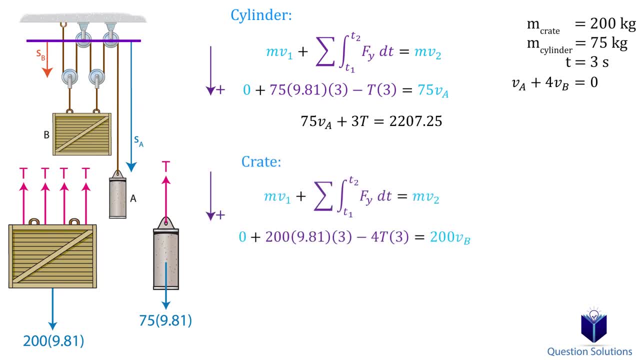 on to the next equation, which will be for the crate. So the initial momentum is zero because the system starts from rest. Then we have the weight of the crate multiplied by 3 seconds. Then we have the tension of 4 cables multiplied by 3 seconds. All of that. 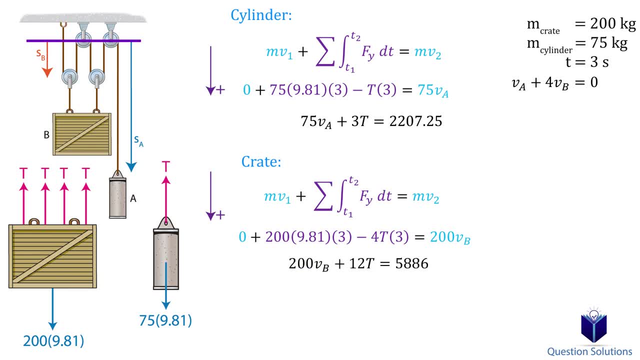 is equal to the mass times velocity. Let's simplify this equation as well. Let's also not forget the equation we found first. Now we have three equations with three unknowns. You can solve them any way you like. We see that we get a negative velocity for the crate. That simply means: 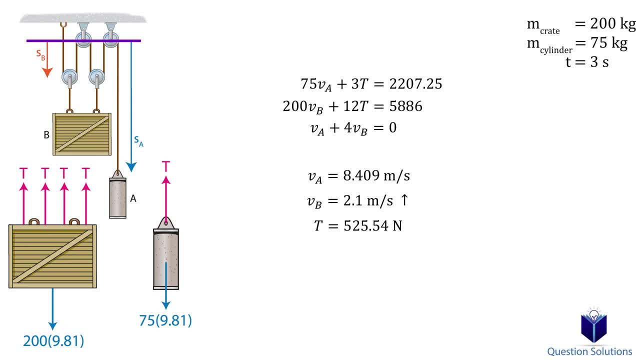 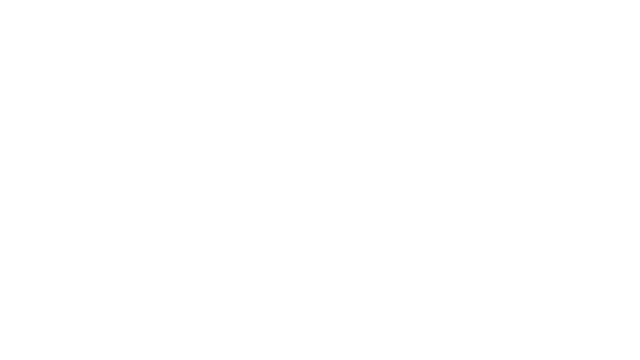 it's going up instead of down, like we assumed. Those are our answers. This should cover the types of problems you will face in this chapter. Thanks for watching and I hope this video helped and wish you the best of luck with your studies. you.